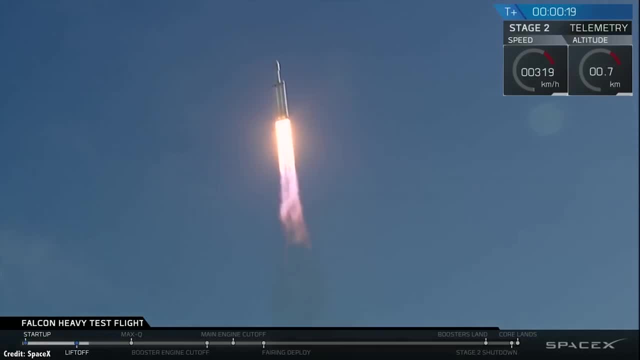 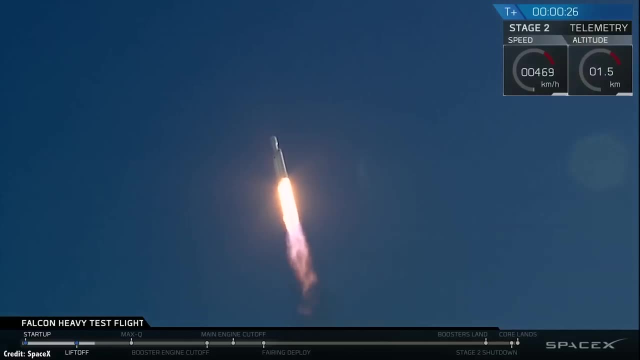 they bring their own oxidizer with them. they work in the atmosphere and they work in the airlessness of space. The advantage of rockets is that they can deliver enormous amounts of energy in short periods of time- the kind of reaction you need to blast tons of cargo. 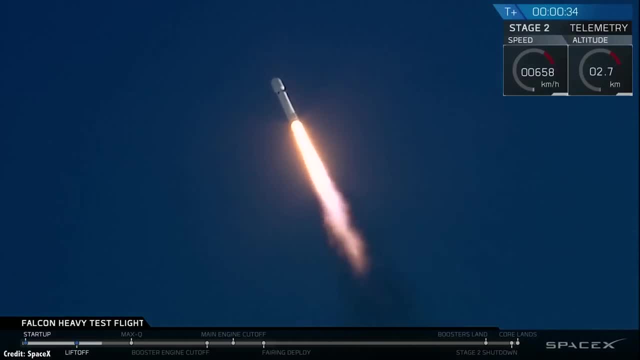 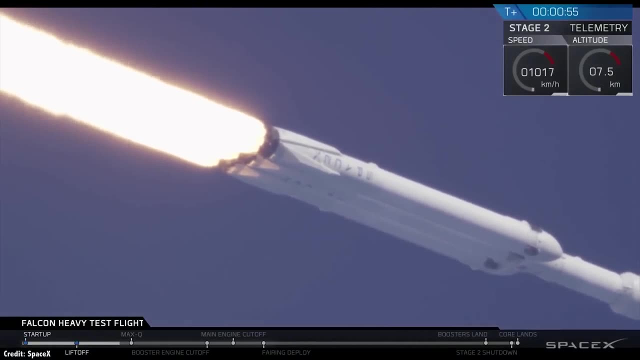 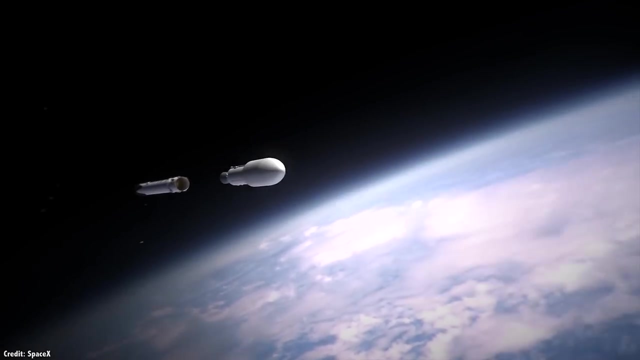 off Earth and into space, but they're incredibly inefficient. A 550 metric ton Falcon Heavy is carrying almost 400 tons of fuel and oxidizer. The first stage will only burn for 162 seconds and the second stage will fire for 350 seconds. 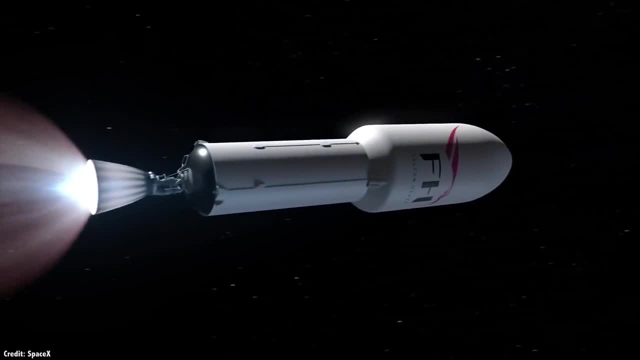 And the second stage will fire for 350 seconds And the second stage will only burn for 150 seconds And the second stage will fire for 300 seconds And the second stage will fire for. That gives you a total burn time of about 9.5 minutes. 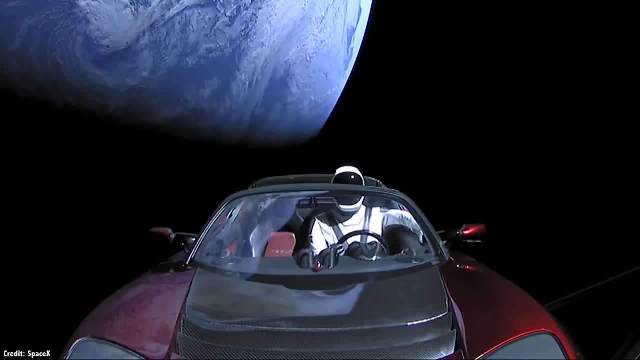 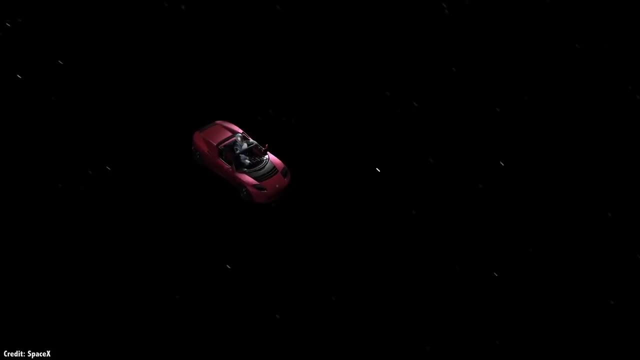 Want to make some maneuvers, Want to accelerate for days, weeks or even months. Too bad, you're out of fuel. Of course, these shortcomings from chemical rockets have led scientists to search for other forms of propulsion, especially when you're out in space, and one of the most 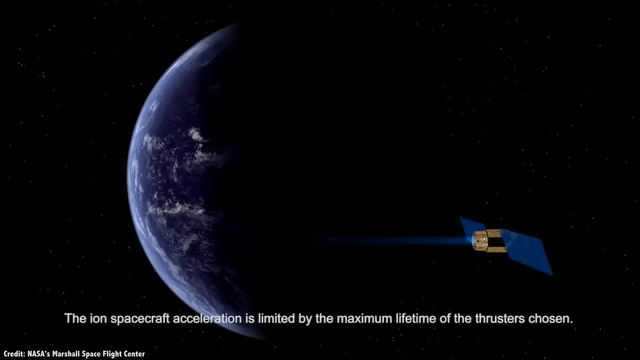 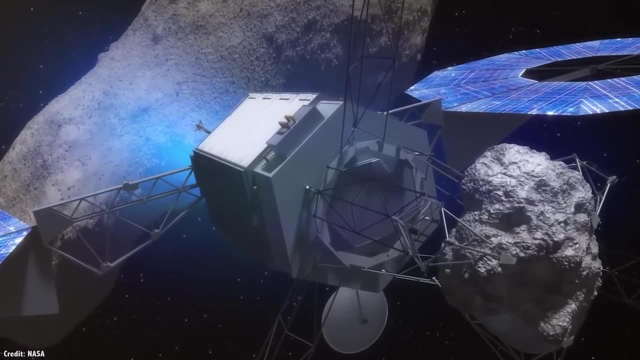 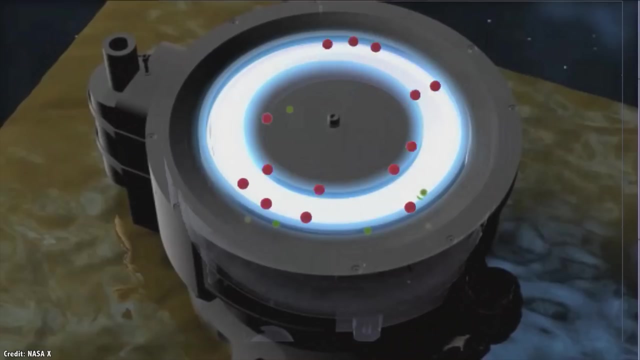 successful so far is the ion thruster. When you're working out the rocket equation, an important factor is the velocity that you're ejecting your propellant. The most efficient chemical rocket can throw hot gases out the back at 5 km per second. 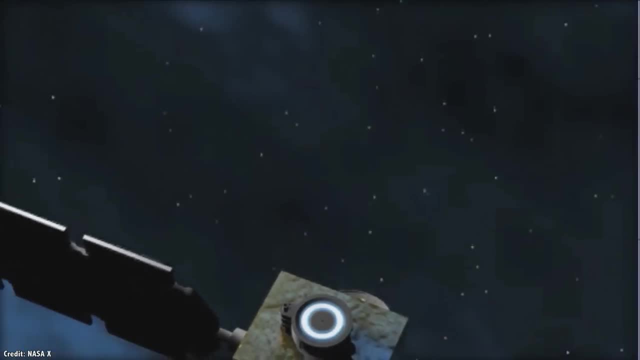 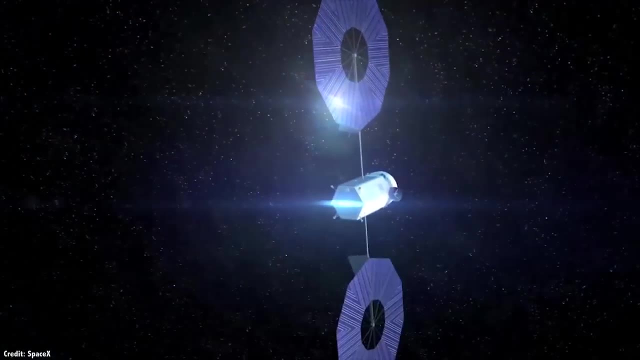 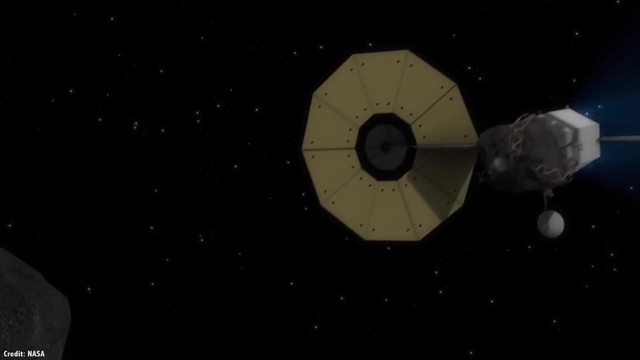 Ion engines, on the other hand, can eject individual atoms 90 km per second. This high velocity gives the spacecraft a much more efficient acceleration. The best chemical rockets see a fuel efficiency of about 35%, while ion engines see an efficiency of about 90%. 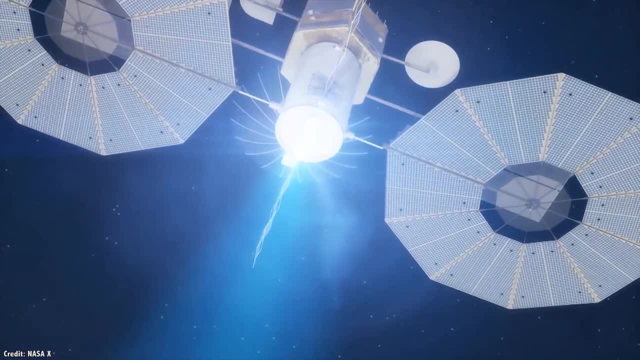 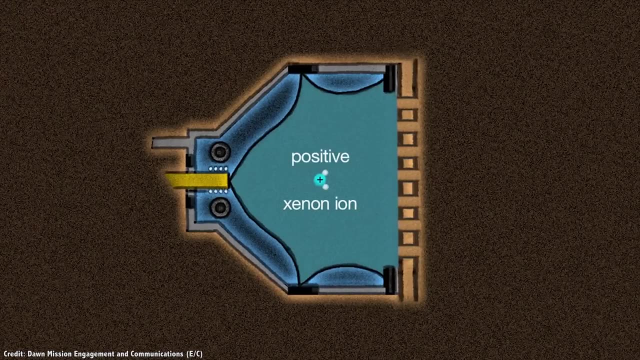 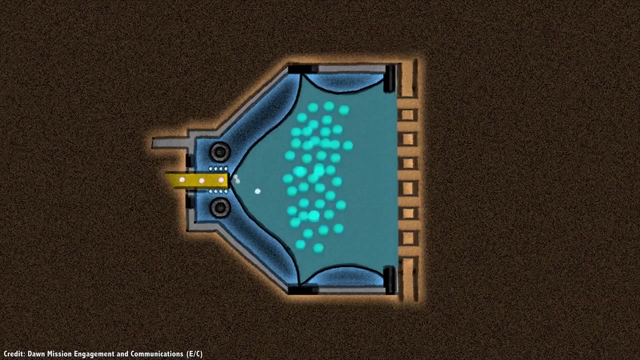 So how do ion thrusters work? It's actually pretty weird and totally sounds like science fiction. Instead of hot gases, ion thrusters eject ions, which are atoms or molecules which have an electrical charge because they've lost or gained an electron. In the case of an ion engine, they're emitting positively charged ions which have lost an. 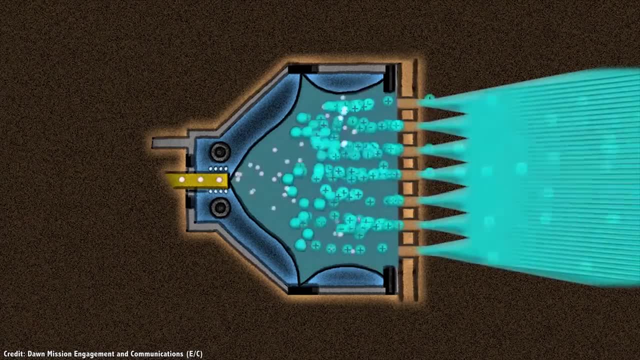 electron. Once you've got ions, you can direct them with a magnetic field, crank them now or gauge делает a motion time, which you can do by essentially reading what the electron resistance field means. see the peak material be the interfering end for the previous system. 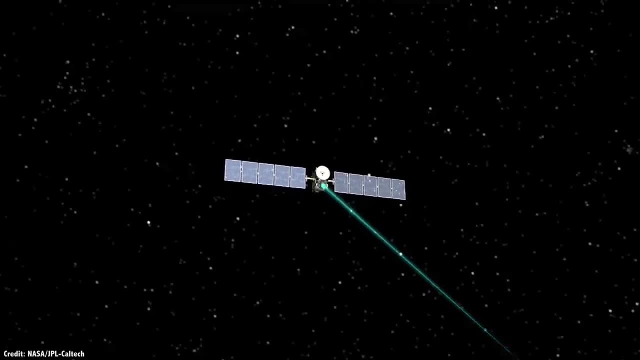 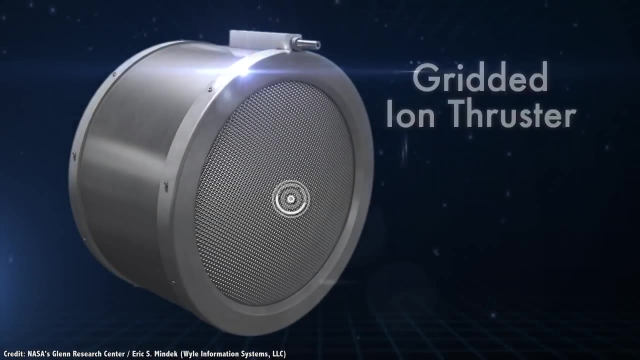 Ok, let's start with the initial structure of the reactor. Be sure to be sure to measure the CO2 concentration field, accelerating them into space at tremendous speeds. So where do they get all the ions? The thrusters create them by generating a plasma inside the spacecraft and they bombard. 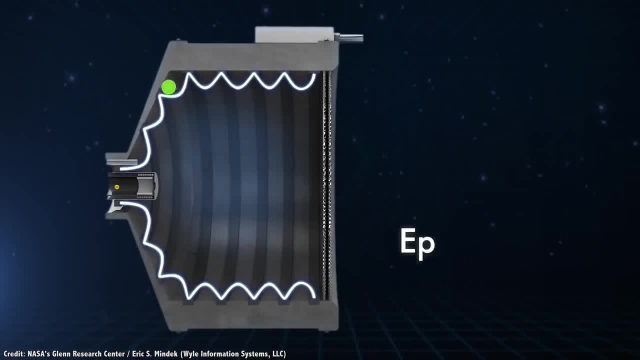 neutral propellant atoms of some gas like xenon with electrons. These collisions release even more electrons from the propellant, turning them into positively charged ions. This plasma soup of electrons and positively charged ions has an overall neutral charge. The electrons are held in the chamber, leading to more ionizing events, while the positive 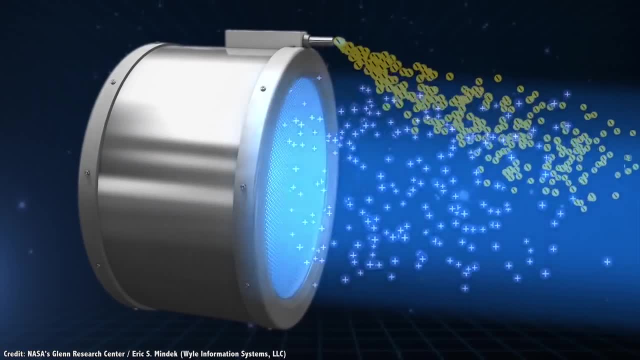 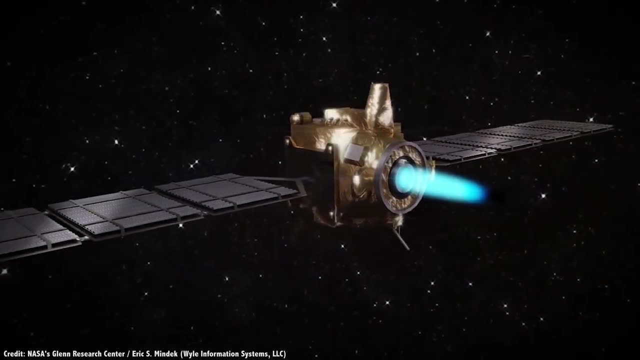 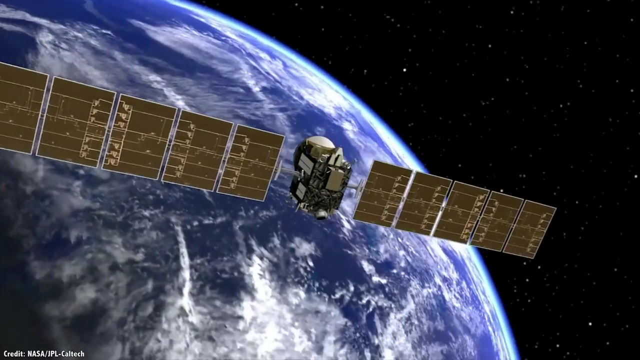 ions are siphoned out through a grid at the end of the chamber. As they pass through this grid, high voltage accelerates them out the back of the spacecraft at speeds of up to 90 km per second. For each ionized particle that the spacecraft can kick out, it gets a tiny kick in return. 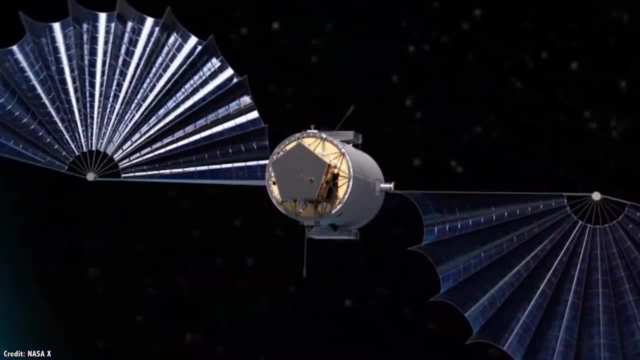 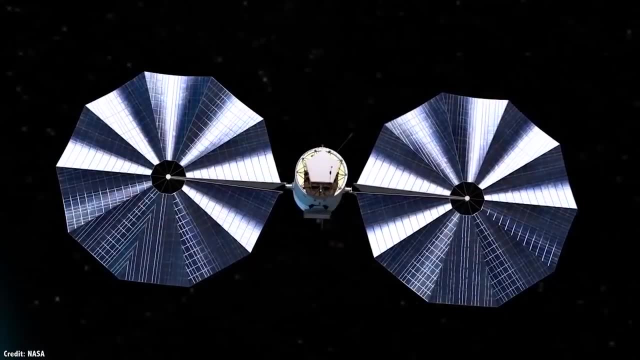 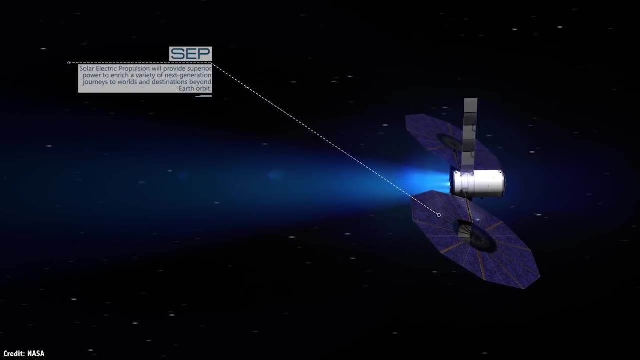 The whole system is powered by solar panels, so the spacecraft itself doesn't need to carry any kind of battery or power system, minimizing the total weight it has to carry. The big problem is that the kick really is tiny. The thrust of ion engines is measured in millinewtons, like thousandths of a newton. 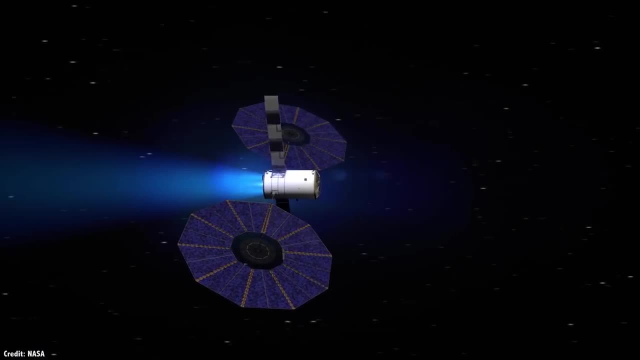 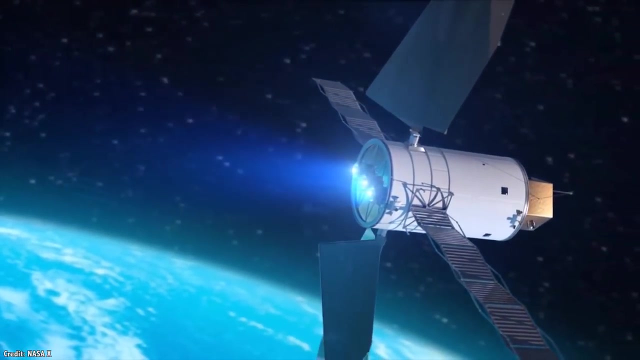 Hold a piece of paper in your hand. that's the kind of forces involved. But they can operate for days, weeks, even months, Accelerating and accelerating Long after chemical rockets would have run out of fuel. So if you're already out of the gravity well of a planet, they're very efficient engines. 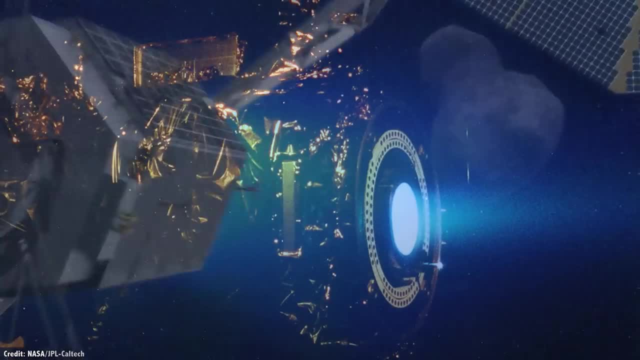 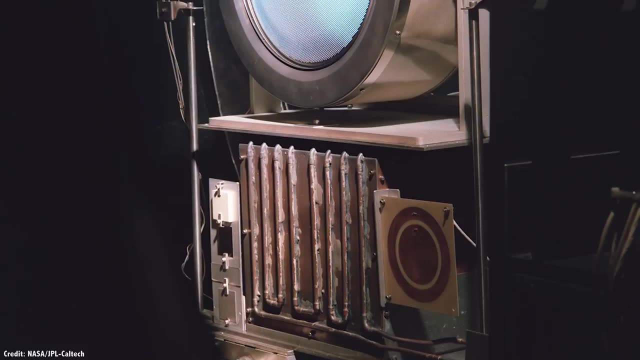 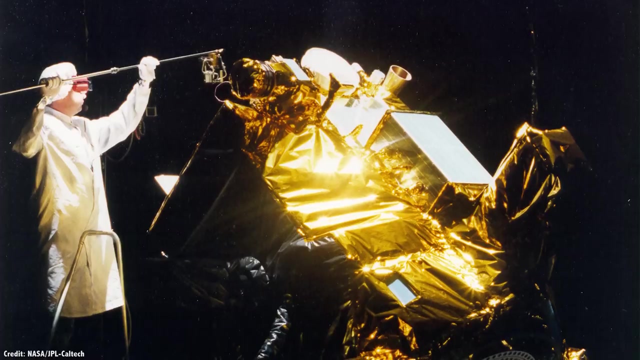 for dramatic changes in velocity. NASA and other space agencies have actually used ion engines very successfully in a range of missions. They've been developing this thruster concept for decades but were never willing to risk it on an active mission where a failure could end it. 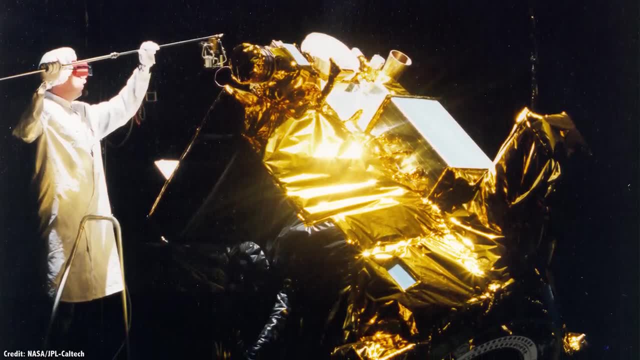 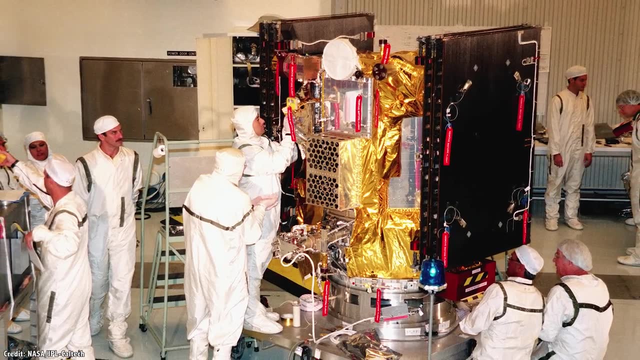 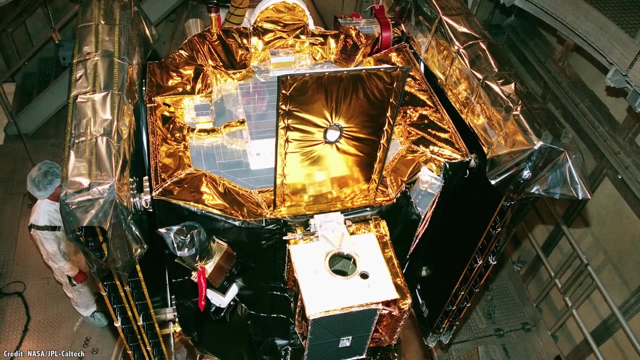 So NASA gathered up a bunch of these risky technologies and packaged them together as the Deep Space One mission, Which launched in 1998.. Deep Space One was equipped with 12 different technologies that NASA wanted to test out, including low-power electronics, solar concentrator arrays, various scientific instruments and 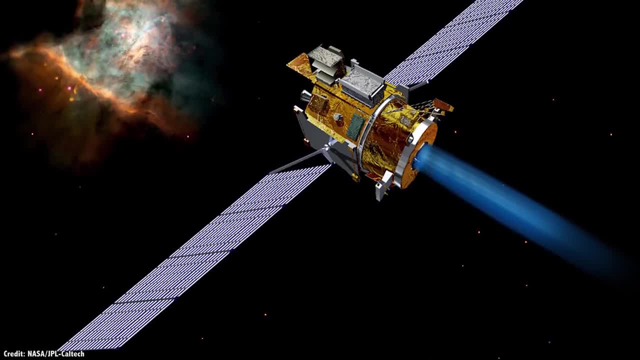 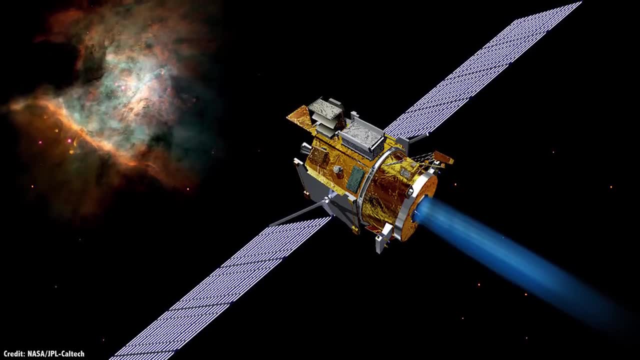 a solar electric propulsion system. Its engine was run for enormous lengths of time, allowing it to make close observations of asteroids and comets, and even Mars. NASA doubled down on the technology of Deep Space One. NASA was able to use the technology of the Deep Space One mission to launch its Dawn. 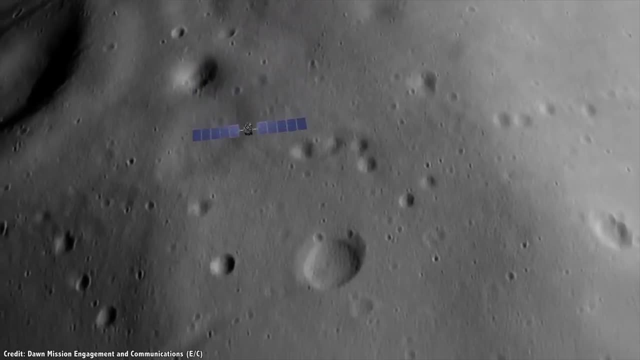 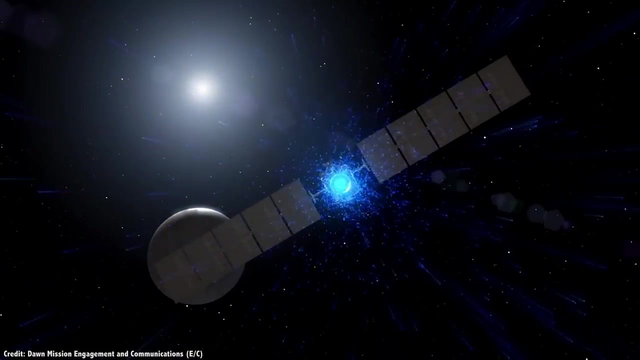 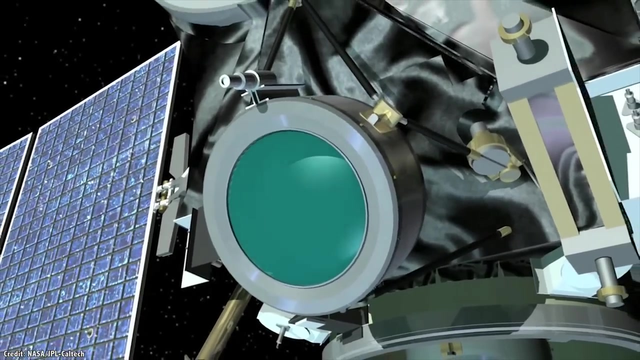 mission three redundant ion engines. These allowed the spacecraft to go into orbit around the asteroid Vesta, make observations, then break orbit and travel to asteroid Ceres and make even more observations, and it could still have fuel in the tank to visit even more asteroids. 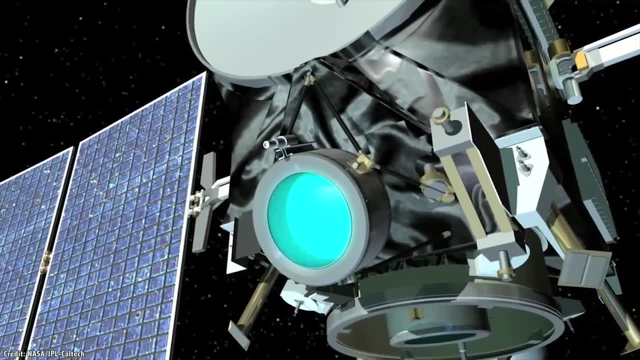 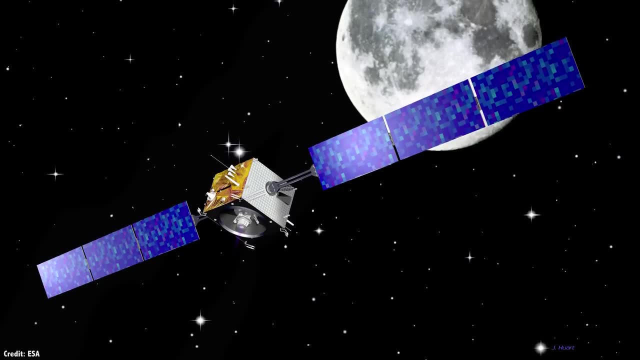 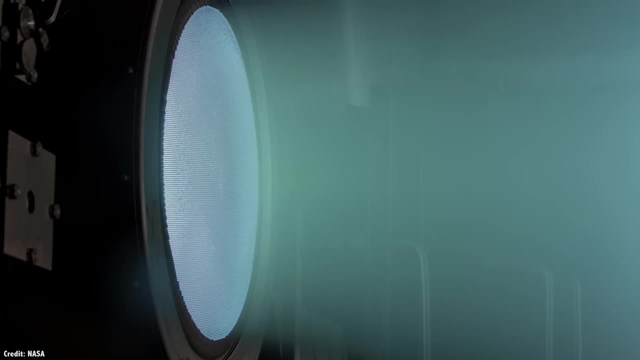 Just to give a sense of its acceleration: Dawn can go from 0 to 100 kilometres per hour in four days of continuous thrusting. Ion thrusters were used to carry ESA's Smart One spacecraft. Ion engines have been tested here on Earth and successfully operated for more than five. 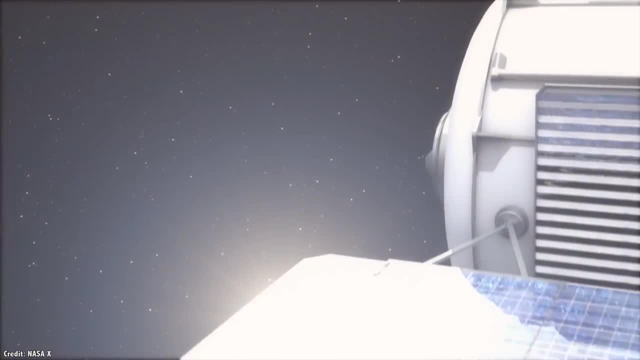 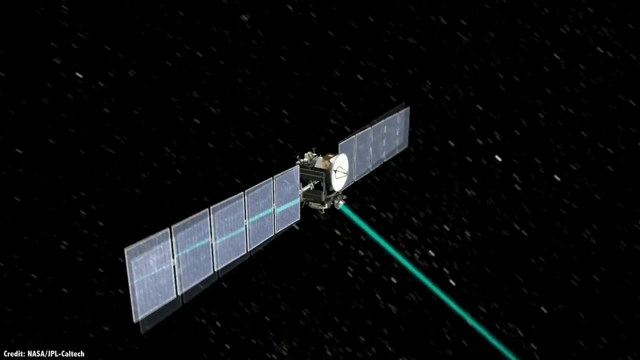 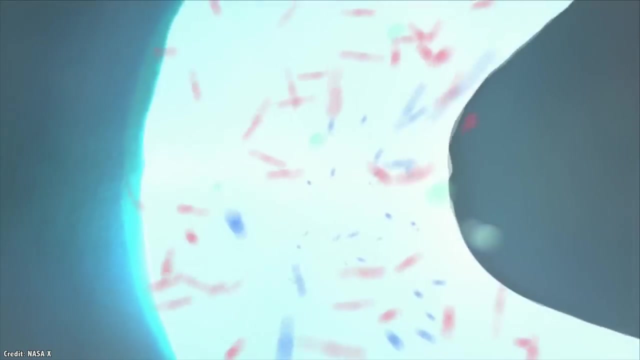 years, continuously With these successes. we're going to see even more spacecraft equipped with ion thrusters in the future, But ion thrusters themselves are getting more powerful and resourceful. I said that ion engines produce very little thrust, But there are some ideas to build them. 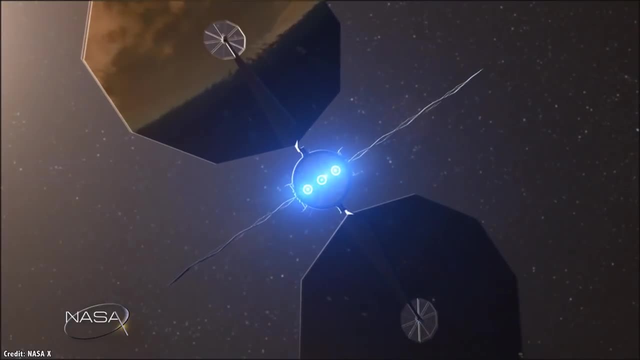 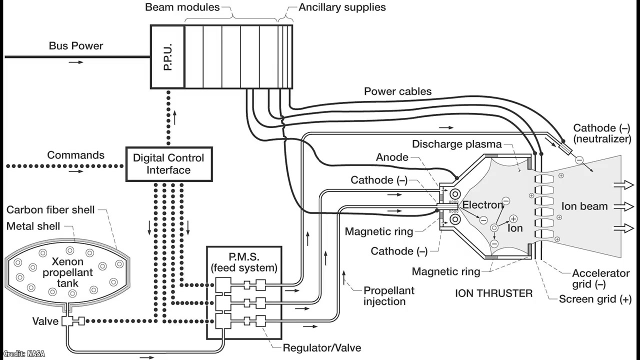 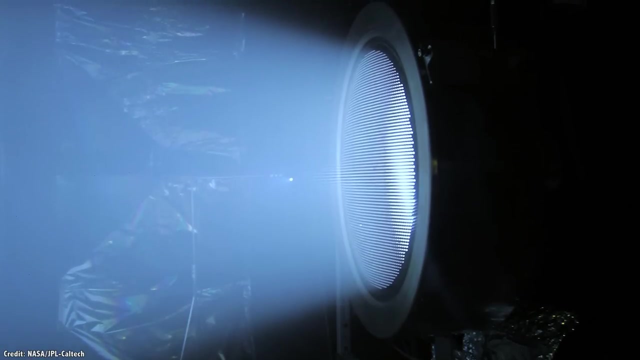 The first is to dramatically increase the amount of electricity you're using to accelerate the ions. Instead of solar panels, NASA considered creating an ion engine powered by a nuclear reactor. About 15 years ago, NASA considered a mission known as the Jupiter Icy Moons Orbiter Mission. 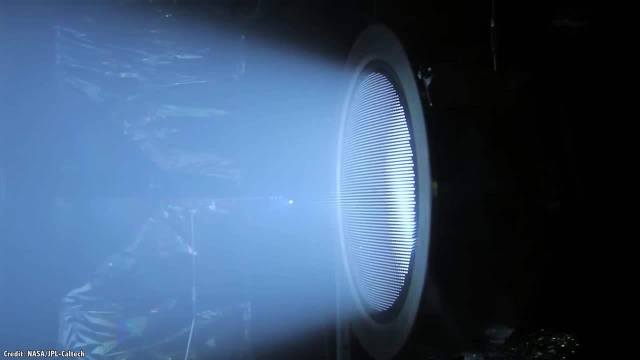 Powered by the Nuclear Electric Xenon Ion System, or NEXUS engine, the spacecraft would be capable of exploring each of Jupiter's icy large moons in sequence. The spacecraft would be capable of exploring each of Jupiter's icy large moons in sequence and would be able to create a nuclear reactor. 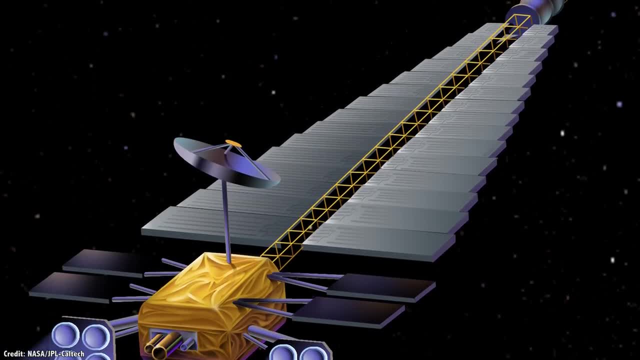 The spacecraft would be capable of exploring each of Jupiter's icy large moons in sequence and would be able to create a nuclear reactor. If I should go into more detail, it can't be improved. The spacecraft would have been launched into orbit in 3 separate pieces, which would then 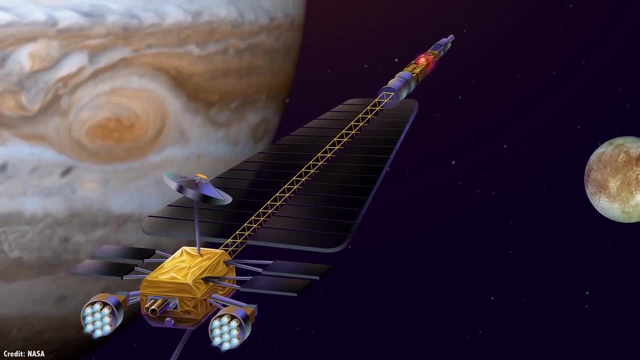 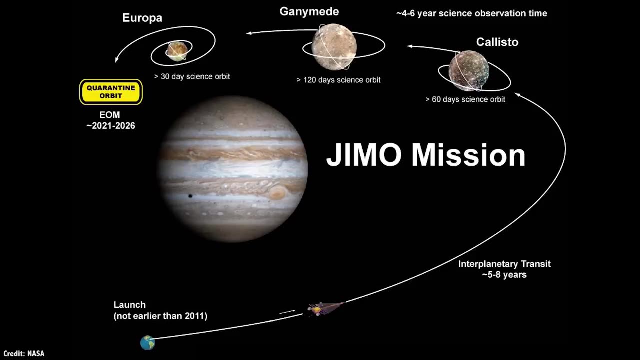 be assembled into Earth orbit and launched off to Jupiter. The spacecraft would use its 8 ion thrusters to study Callisto, then Ganymede for 3 months each and then settle into a final orbit around Europa. If conditions were right, it could even go into orbit around Io. Of course, we don't get to have nice things, and the mission was cancelled back in 2005.. There are other ways ion thrusters can be scaled up. NASA is testing a high thrust version of ion engines known as the X-3 Hall Thruster.